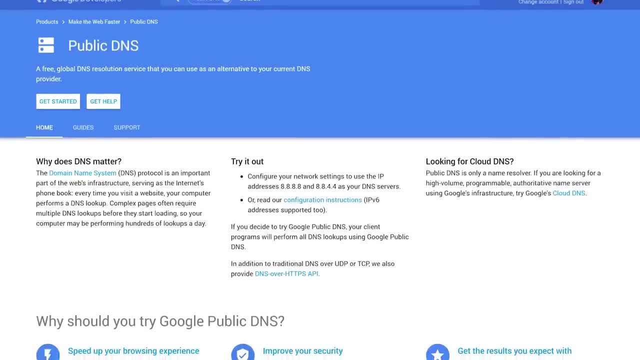 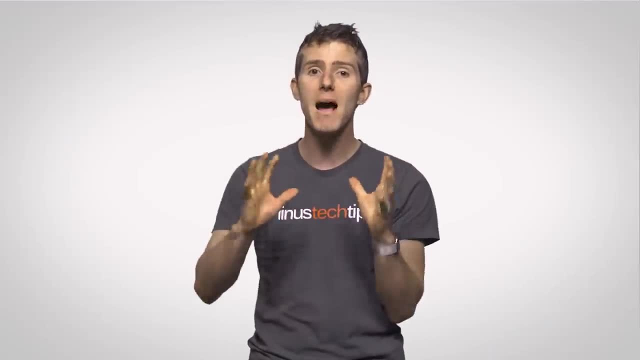 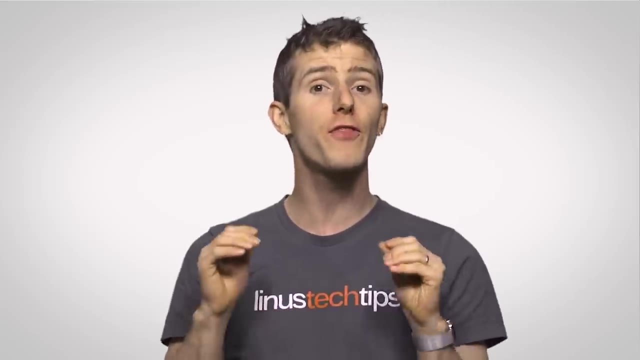 but you can also use public servers managed by Google or other organizations. if your ISP's resolver is having issues, A recursive name server might have the IP address of the website you want to access already stored, but if it doesn't, it will go to one of 13 root servers which manage requests for top-level domains like 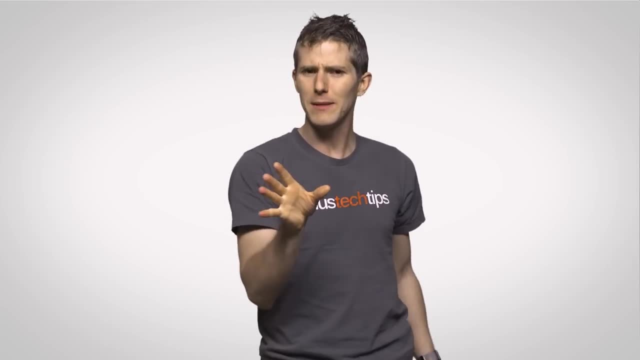 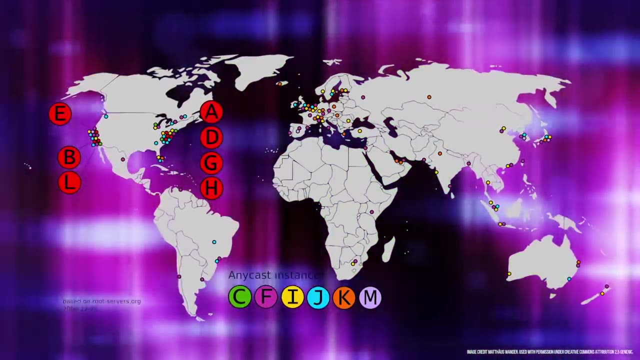 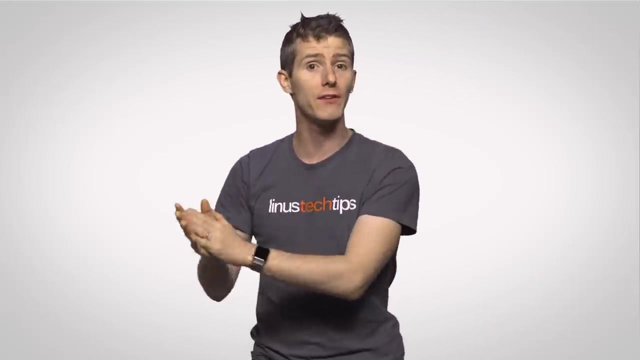 com or org, Although that seems like a tiny number of servers. by the way, they actually use redundant physical hardware all over the globe to make sure these requests are handled, and handled quickly. Your request is then sent to the appropriate top-level domain server- com, if you're trying to get to YouTube, for example- which will then contact. authoritative name servers that contain a well authoritative list of IP addresses and matching URLs, which is updated whenever someone buys and registers a domain. Once the IP address you want is retrieved, it's sent back to the recursive name server and then on to your computer. To save time in the future and make things more efficient. 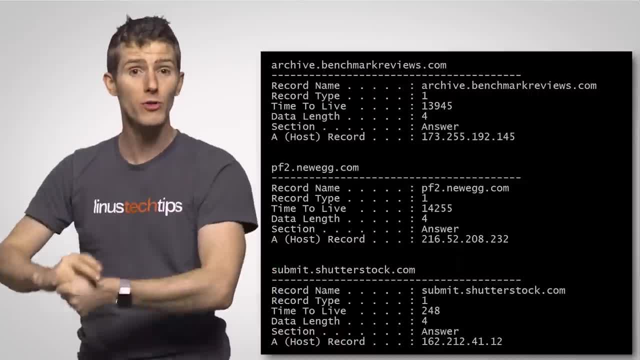 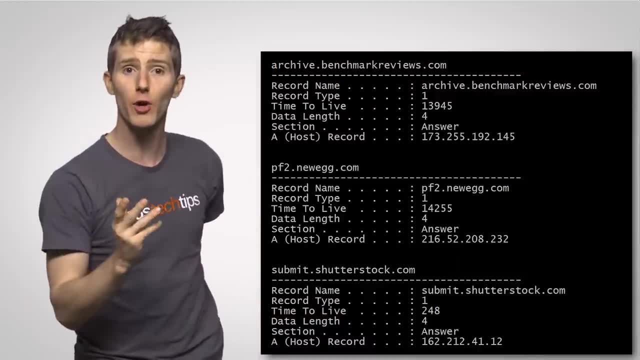 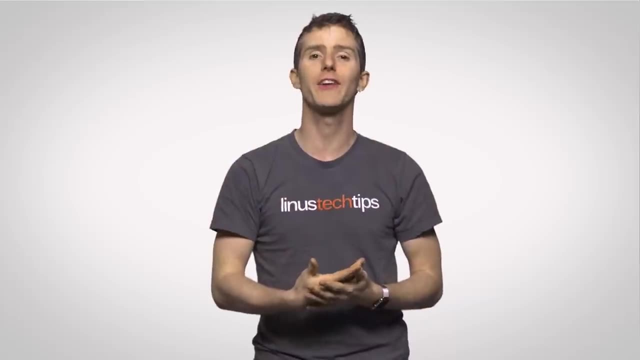 both the recursive name server and your own computer will cache DNS entries for a while, so the next time you want to visit YouTube, you won't have to go through this whole rigmarole. Instead, your computer will either know the correct IP right away or it will be able to get it directly from the recursive server. 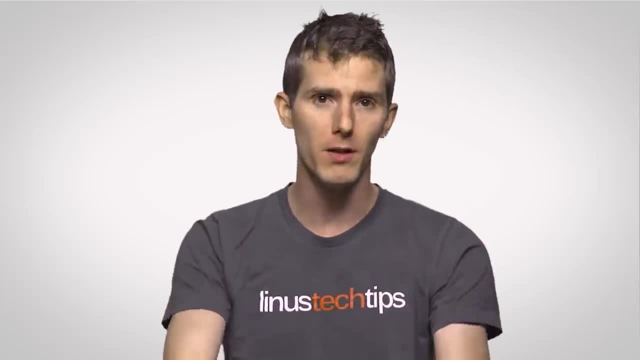 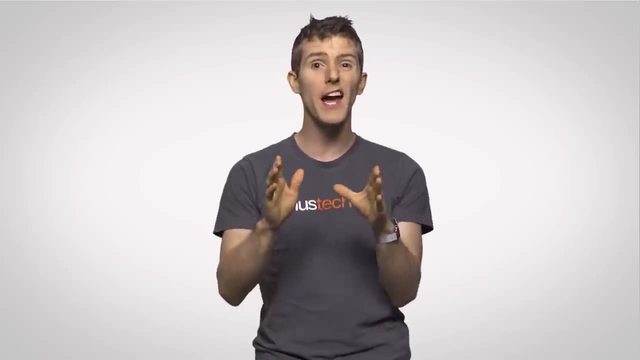 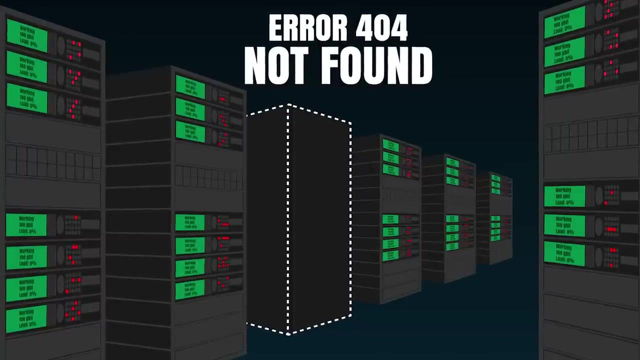 DNS usually works fairly well for most people, but if a website changes IP addresses, this can cause problems, especially if your computer is trying to use its own cache. This will usually manifest as lots of random 404 errors or taxi drivers taking you to the wrong place. if we were to harken back to our original analogy, So if you're running Windows, it's actually pretty easy to clear out your DNS cache just by opening the command prompt as an administrator and entering this command, which hopefully will fix the problem. However, you could run into more serious problems if a piece of malware has poisoned your DNS cache by making DNS entries that are stored locally. 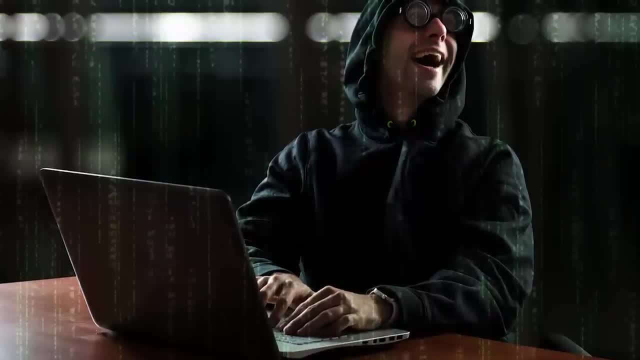 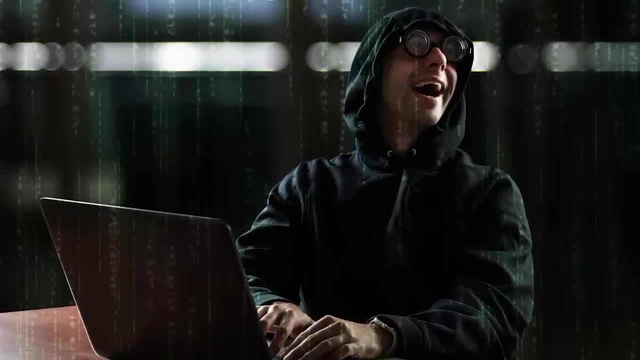 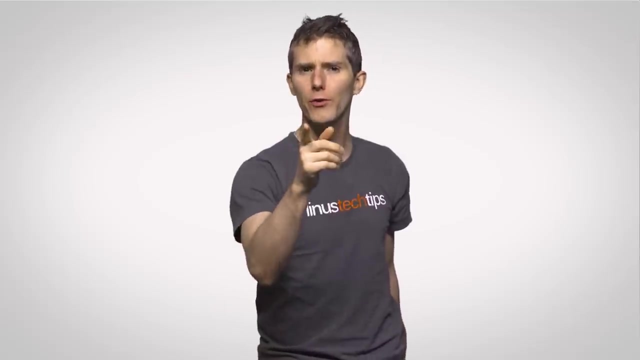 that point to malicious websites. For example, an attacker could tell your PC to make irsgov point to the IP address of a website running a tax scam that tries to convince you to give up your personal information. So if you're getting weird redirects like this, running, a reputable anti-malware application may be able to fix it. 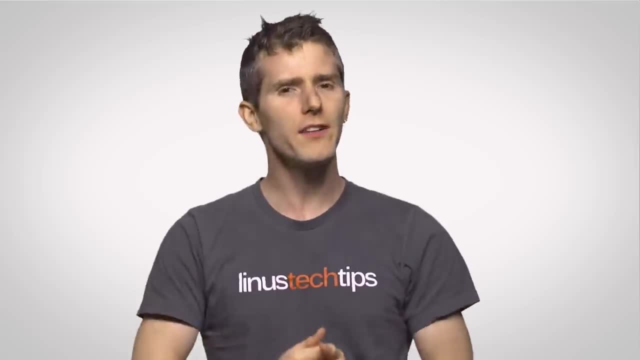 So if you're getting weird redirects like this, running a reputable anti-malware application may be able to fix it. So if you're getting weird redirects like this, running a reputable anti-malware application may be able to fix it, But despite its vulnerabilities. 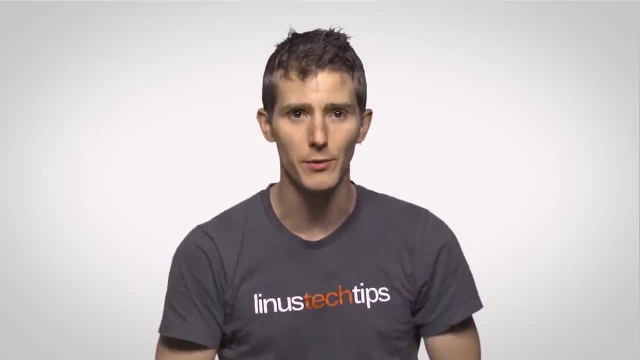 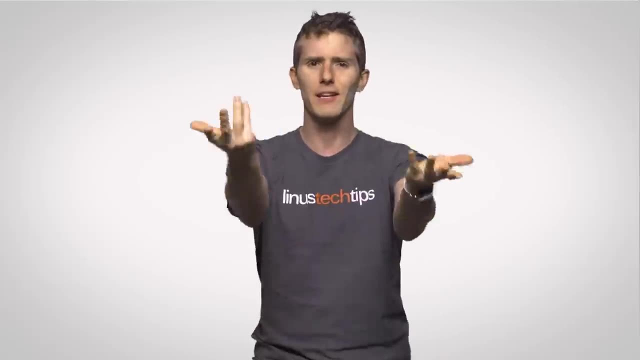 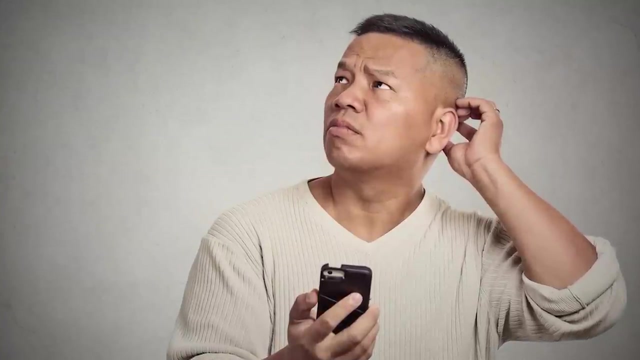 DNS has made the internet extremely easy to use for many people because, thanks to it, we don't have to punch in numerical IP addresses like phone numbers, except longer, every time we want to surf the web, And given how hard it is for people to remember phone numbers,